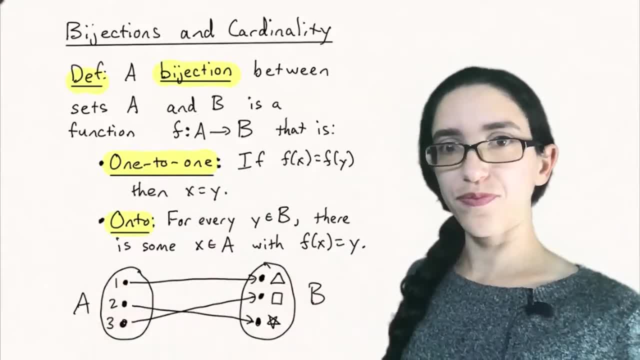 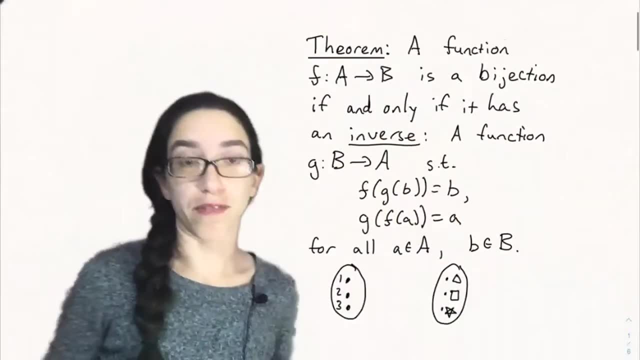 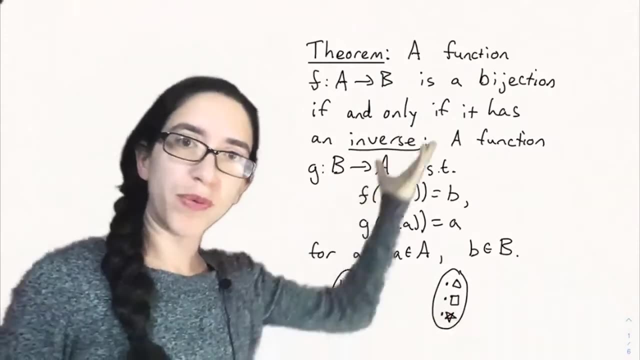 matching between the elements of A and the elements of B. Now let's look at an important theorem about bijections. that's useful in proving a lot of facts about them and also useful in knowing when you have a bijection between two sets. If you have some mapping, when do you know it's a bijection? Well, an easy. 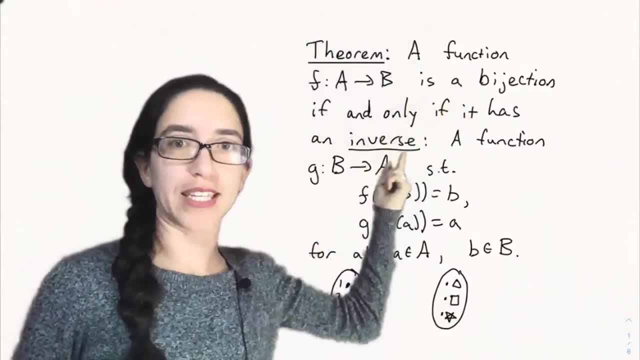 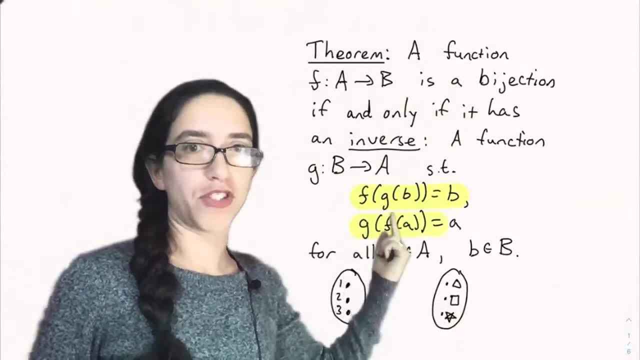 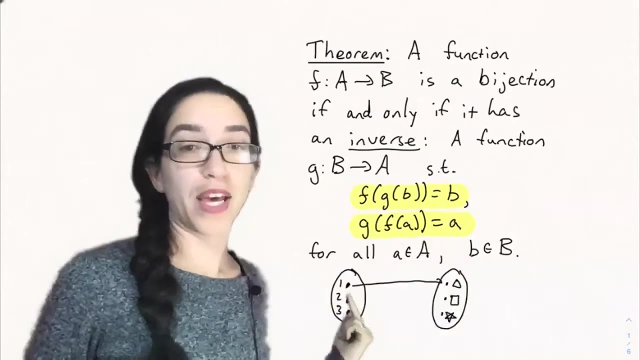 way to tell is that f is a bijection if, and only if, it has an inverse, and an inverse is a function g from B to A that reverses the map. So f of g of B is B for any B in here, and g of f of A is back to A for any A in here. What that means is: 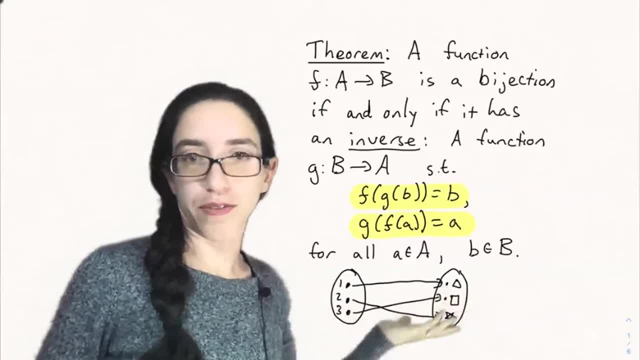 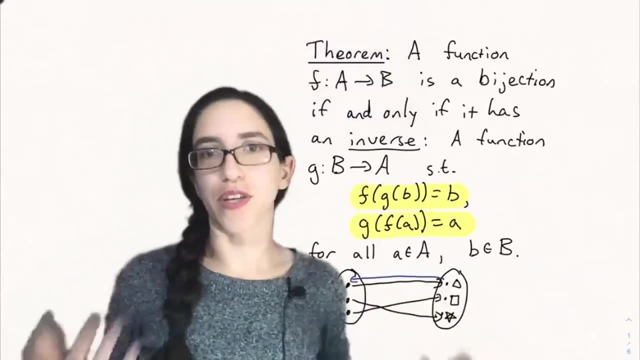 that if you draw it as a diagram of arrows, for these finite sets, for instance, then the inverse is just given by reversing arrows and making them go backwards, And so that's how you can think of the inverse function. It's going to be a function because it's a bijection, and so all. 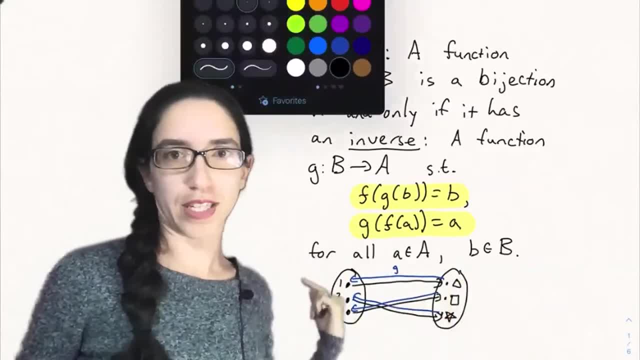 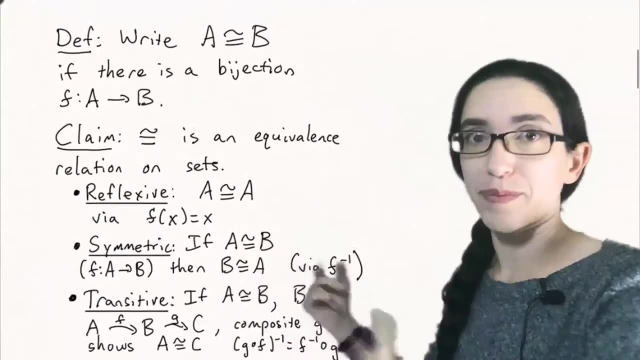 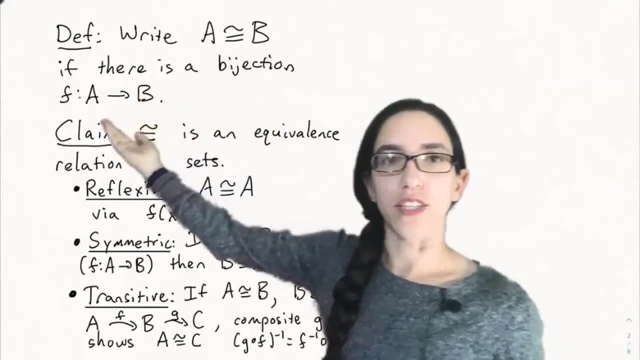 these points have exactly one arrow coming into them, so they have exactly one arrow coming out of them. So this theorem comes in handy for proving things like the following: So if we write: A is equivalent to B, let's define a relation, A is equivalent to B if there's a bijection from A to B, If it's just. 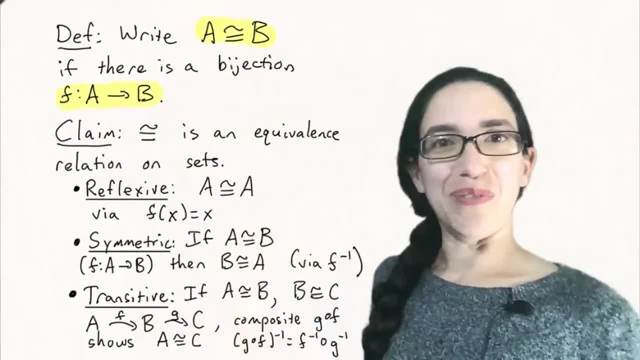 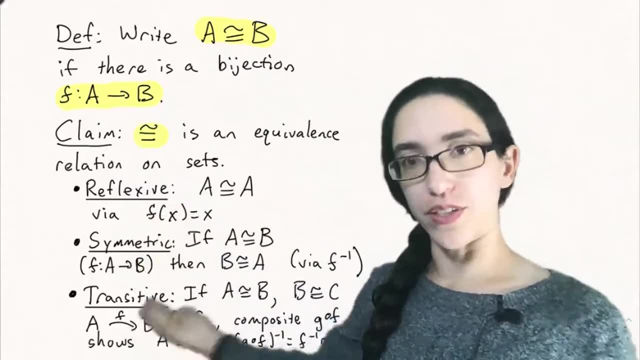 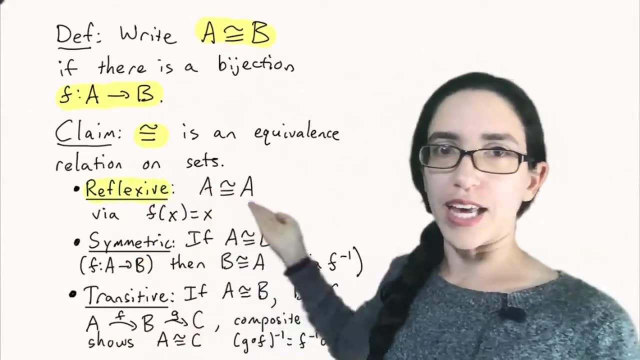 there exists some bijection out there somehow. So then, that relation is actually an equivalence relation on sets in the sense that it satisfies the three properties of equivalence relations that we've discussed before, And those three properties are reflexive, symmetric and transitive. Reflexive says that any set is related to itself, So is there a? 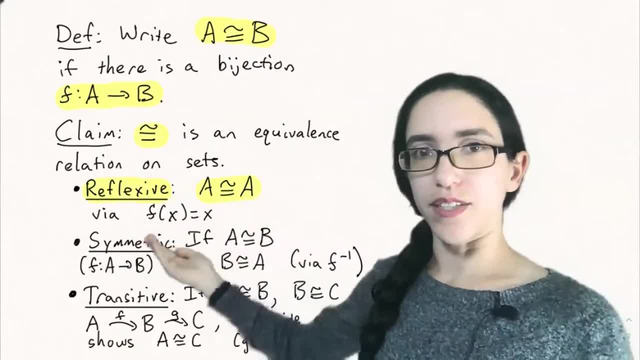 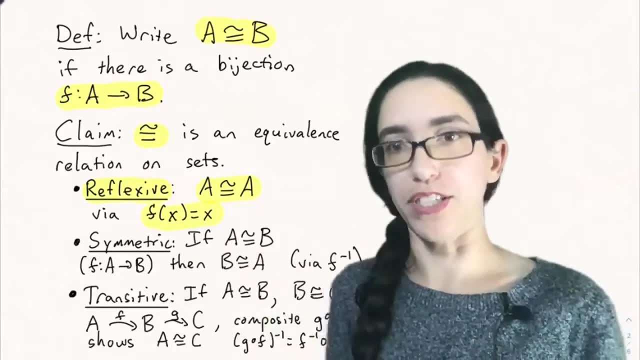 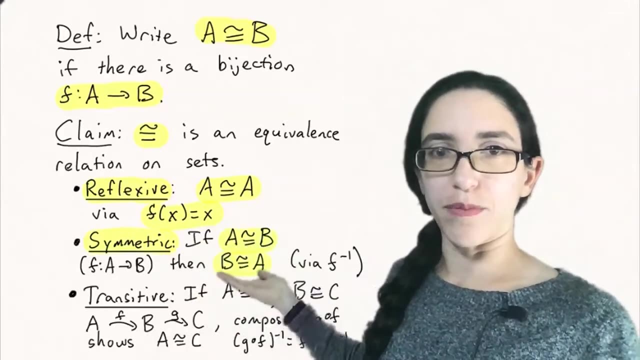 bijection between any set A and itself. Yes, the the bijection that sends any element x to itself. x just goes to x itself, then that's a. that's a bijection, because it inverses itself. So that's your reflexive Symmetric says that if A is equivalent to B, then B is. 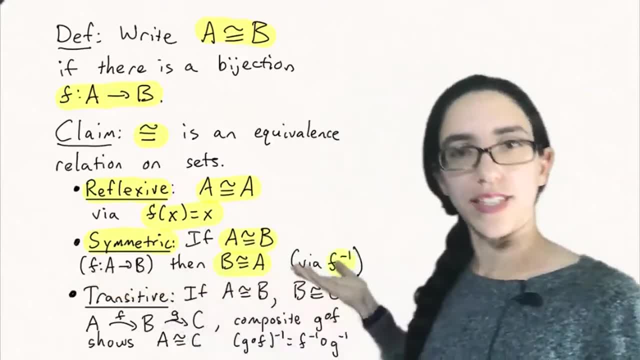 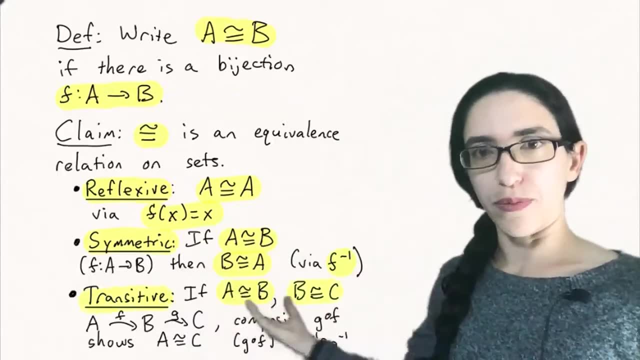 equivalent to A and indeed, if there's a bijection from A to B, then it's inverse is a bijection from B to A. And finally is it transitive. if A is equivalent to B and B is equivalent to C, That means there's a bijection from A to B and a bijection from B to C, and we can. 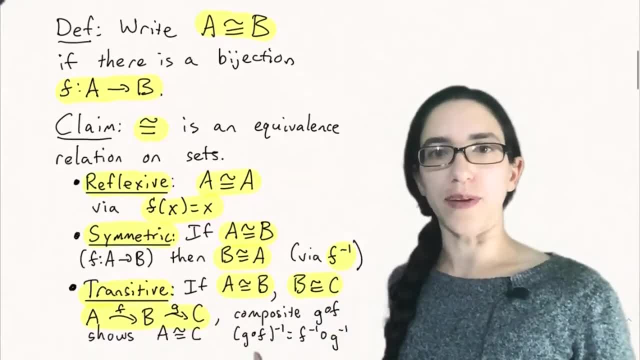 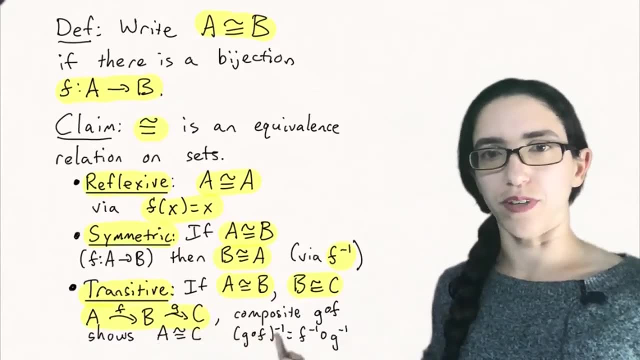 take the composite: just follow the arrows from A all the way to C to get a bijection from A to C, And indeed the inverse of a composite g Jacobi composed with F is what that composite function is called is actually the. 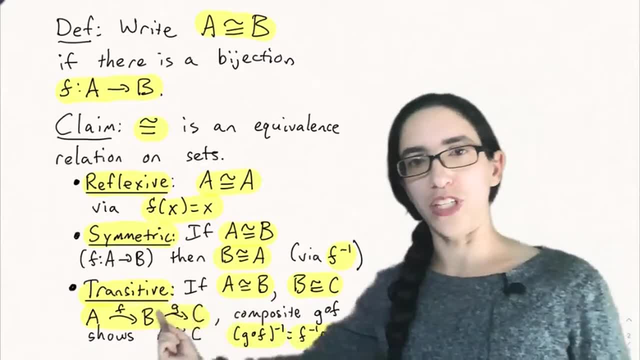 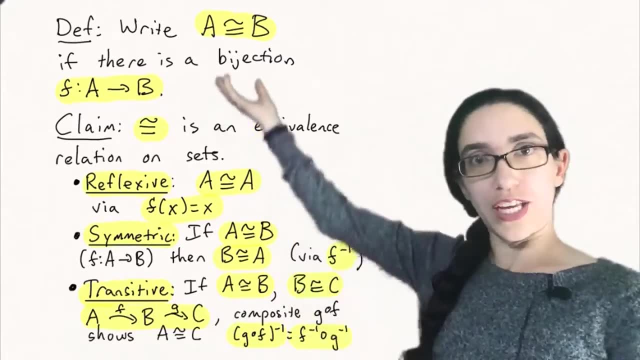 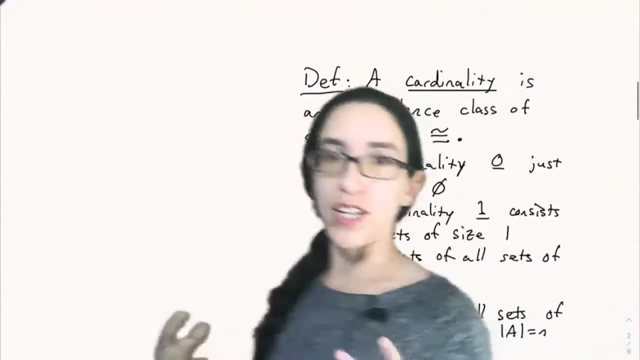 inverse of F composed with the inverse of G, meaning you follow G backwards and you follow the F arrows backwards, and that reverses the whole bijection. So we have an equivalence relation defined by the existence of bijections between sets. And so when we have an equivalence relation, we want to look at equivalence. 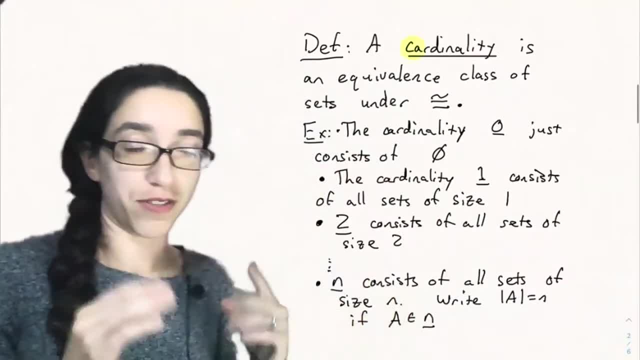 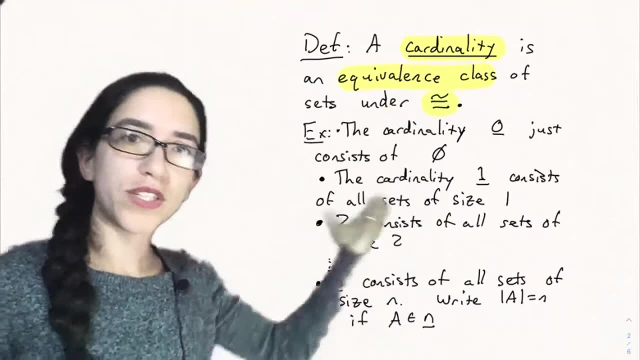 classes And the equivalence classes under this relation are called cardinalities. A cardinality is an equivalence class of sets under bijection. So let's look at some examples of cardinalities. Let's look at the cardinality of the empty set. The empty set is only in bijection with itself and 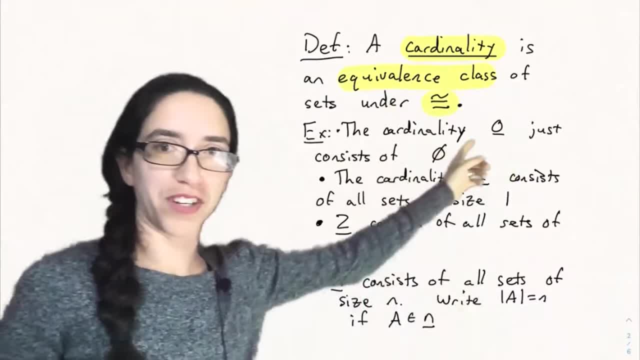 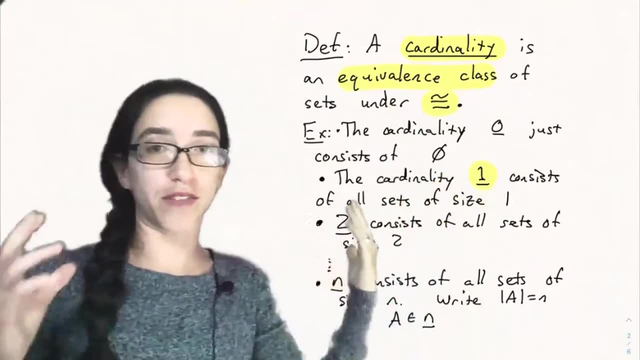 no other sets. So we'll call that cardinality 0, with a little underline to distinguish it from the number 0.. Cardinality 0 just consists of the empty set. The cardinality of 1 consists of all sets of size 1.. That. 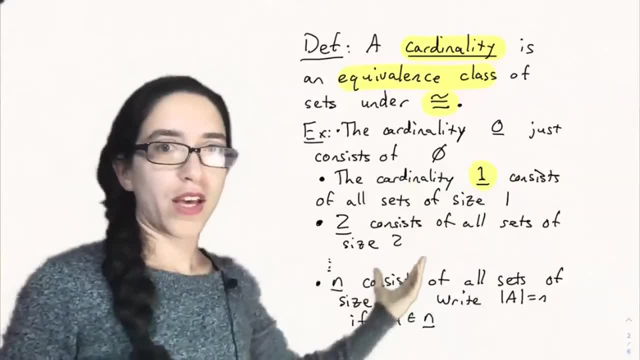 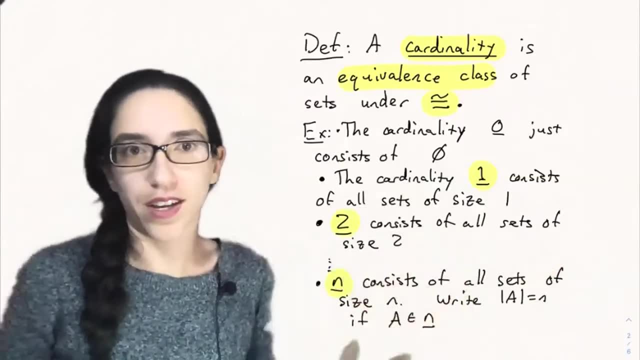 entire class of sets is one cardinality, And similarly, 2 consists of the class of all sets of size 2.. It's an enormous number of sets. Any two things represents the number 2.. Similarly, n is the class of all. 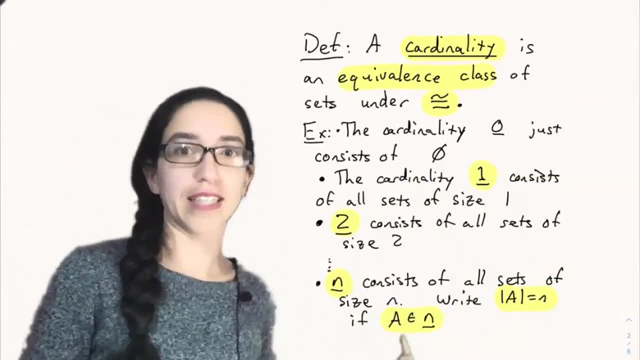 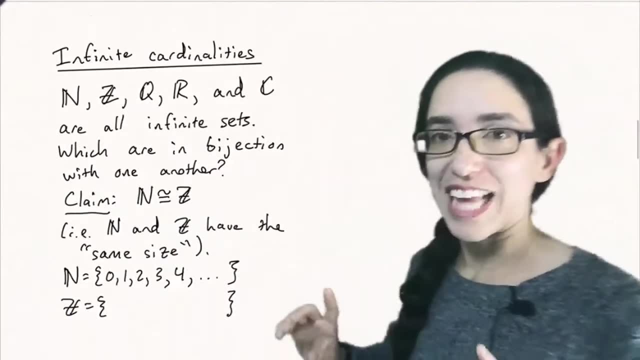 sets of size n and we write: size of A equals n if A is in that cardinality, if it's a member of that equivalence class. So the fun thing here is now we can compare infinite cardinalities, So finite cardinalities is where we do. 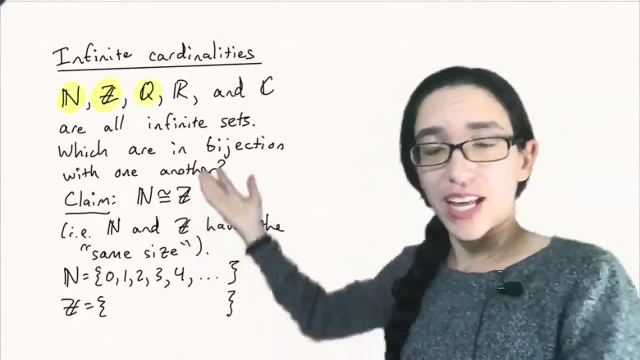 combinatorics to figure out how many elements are in a set, But how many elements are in an infinite set? And let's just look at the cardinalities. We're gonna find out how many elements are in a set And how many elements are in an infinite set. And 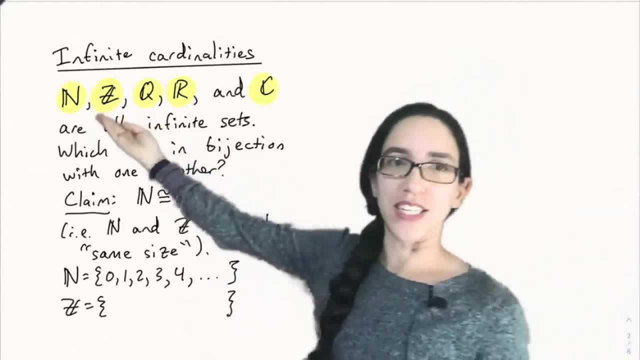 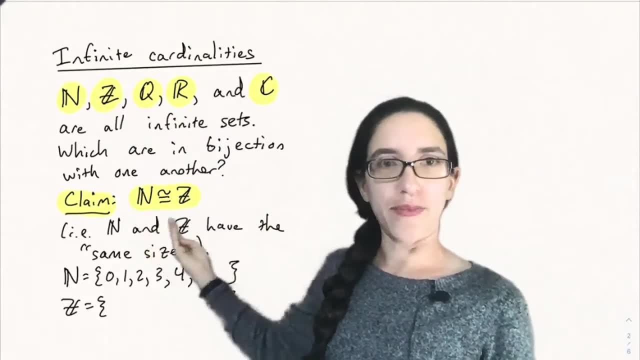 are they different at all from each other? Let's look at the infinite sets n, z, q, r and z, some of our favorite ones. Let's first look at n and z. I claim these are the same size in the sense that. 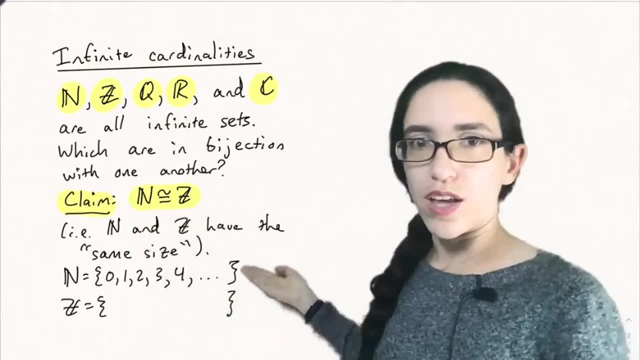 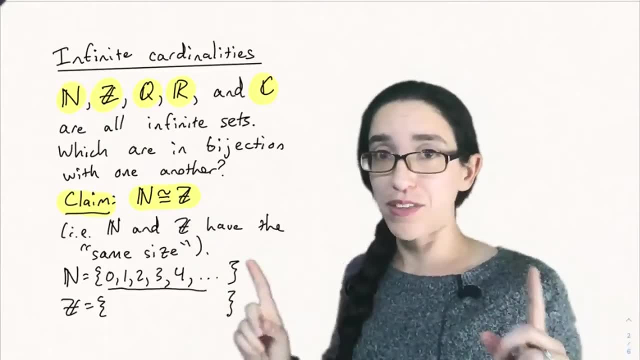 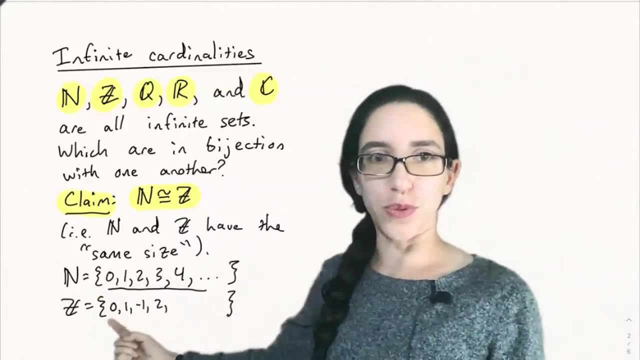 there's a bijection between n and z, So this may seem unintuitive because you'd think the natural numbers are contained in the integers. as a subset, They can't be as big. But strange things happen in infinity. And in fact, in order to make a bijection between 0,, 1, 2,, 3, 4, etc. and the integers, we just 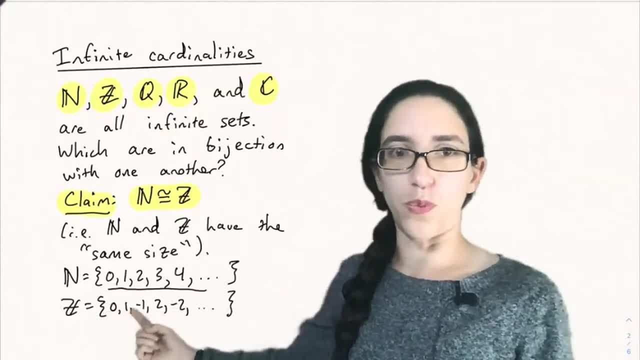 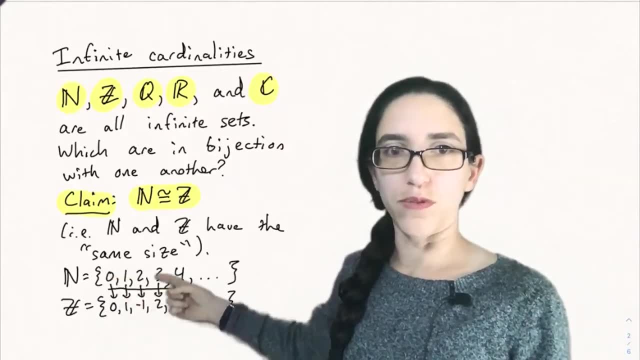 need to list the integers in some order. Let's list them as 0, 1, minus 1, 2, minus 2, 3, minus 3, etc. And just make the bijection by just drawing an arrow from the next number to the next number in. 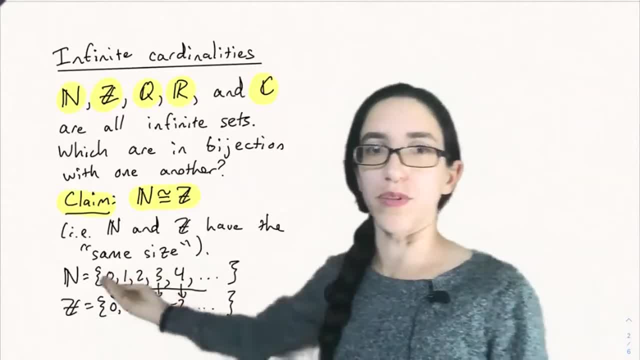 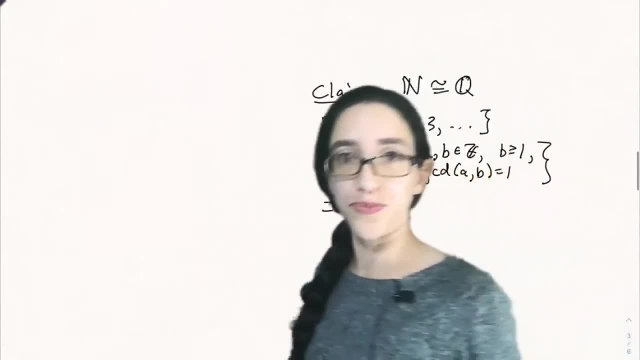 the sequence. So anything that can be listed in order is in bijection with the natural numbers, And z can be listed in order, And so every element of z is in this list, and so it's a bijection. So the natural numbers and the integers are actually the same size of infinity, So we have 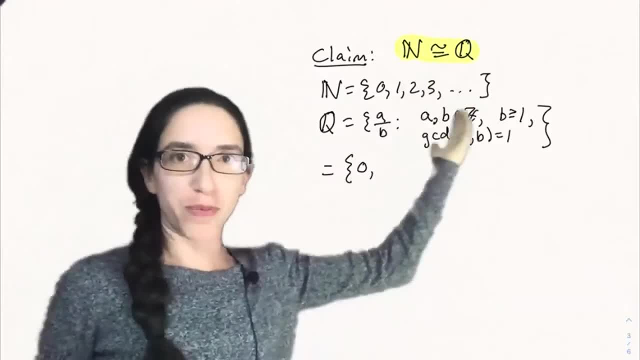 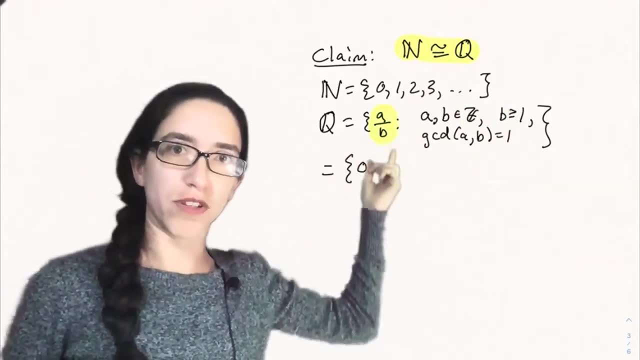 the natural numbers and the rationals, it turns out. So the natural numbers again are 0,, 1,, 2,, 3, etc. the counting numbers And the rational numbers we can write as the set of all a over b. 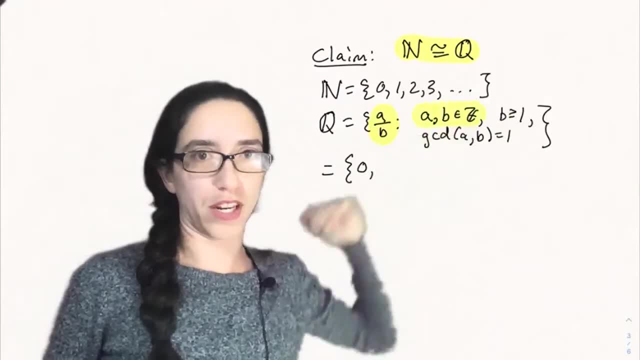 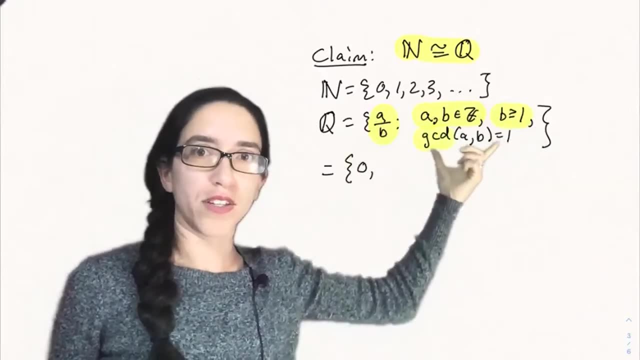 fractions, so that a and b are both in the integers And b is greater than or equal to 1, so that we're not dividing by 0, and the negative sign is always in the a And also gcd of a, b equals 1.. We say: 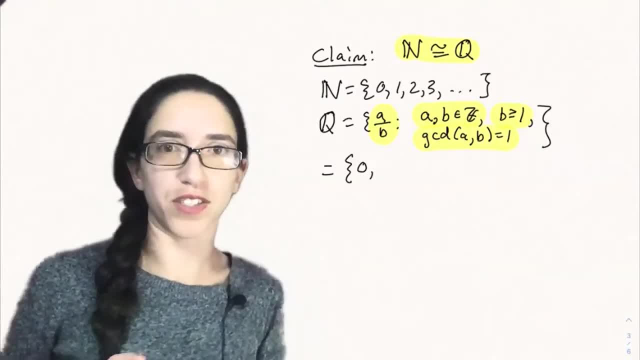 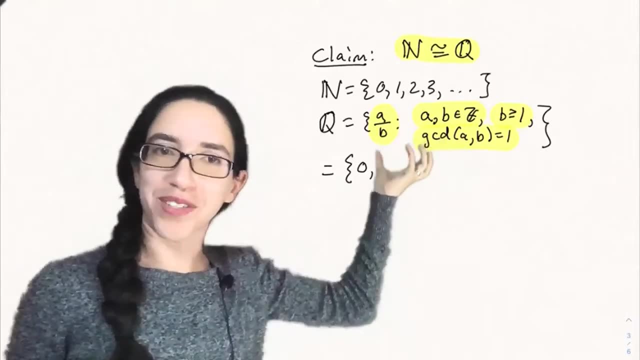 they're relatively prime, just so that we have a reduced fraction. So we're not listing 2 over 4 as different from 1 over 2.. So now can we list all of the elements of the rational numbers in some order? It seems pretty hard, But when we think about it let's start with 0, and let's list them. 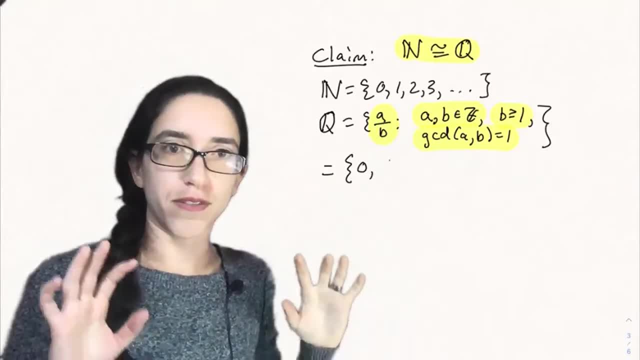 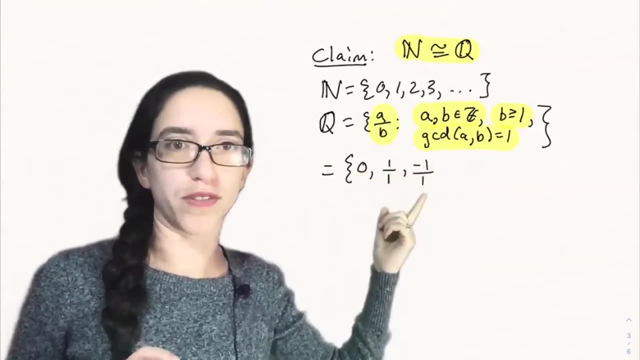 in order of the sum a plus b. Let's first consider the smallest possible sum a plus b can be. That would be 2.. We can have 1 over 1, and then the negative of that as well, just like we did for z. 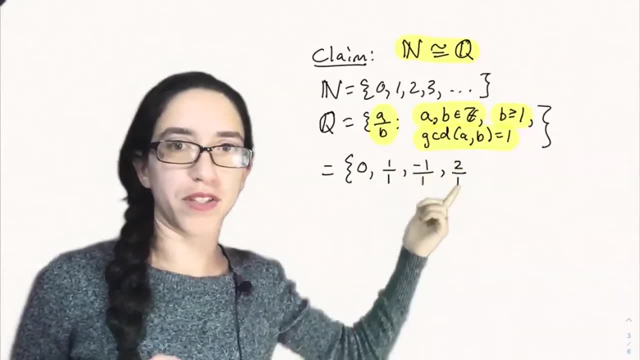 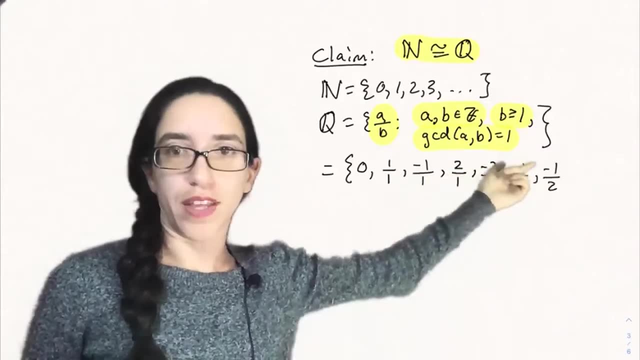 minus 1 over 1.. Now, if the sum of the a and b is 3, we could have 2 over 1, and it's negative minus 2 over 1, or 1 over 2, and then we list it's negative minus 1 over 2.. Okay, that's all the possibilities where a plus b is 3.. 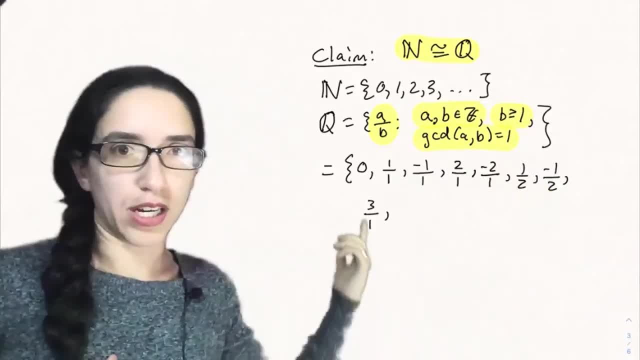 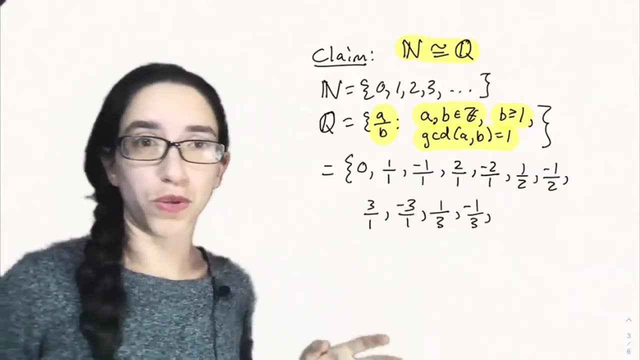 What about if a plus b is 4?? Well, we can have 3 over 1 and minus 3 over 1, you know, just negating 1 over 3 and minus 1 over 3.. We can't have 2 over 2, because that's not reduced, That's the same as 1. 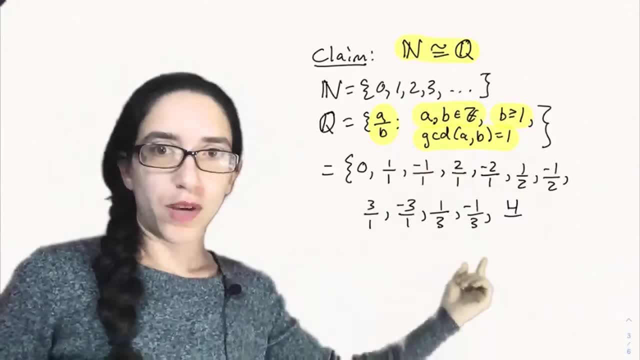 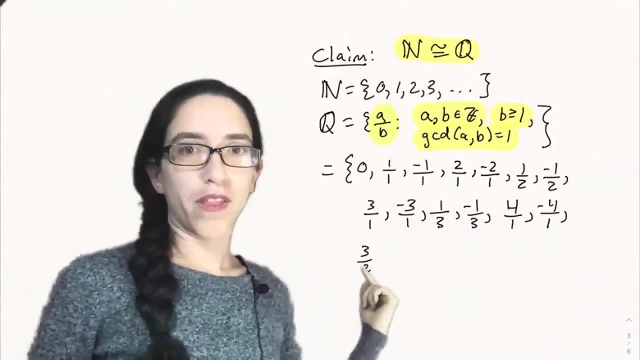 over 1.. We're going to skip that because of the gcd condition. We don't want to list an element twice. after all, For sum equal to 5, we have 4 over 1, and it's negative. 3 over 2, and it's negative, and then 2 over 3 actually does work, so we get more. 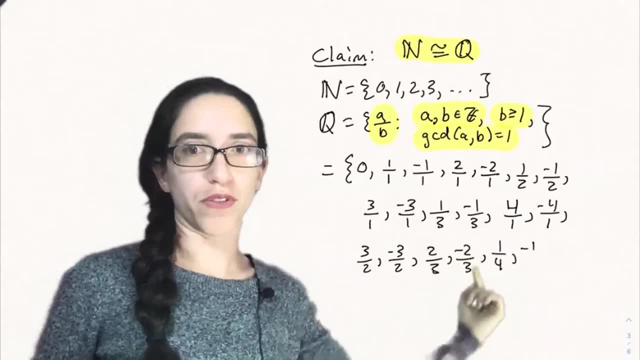 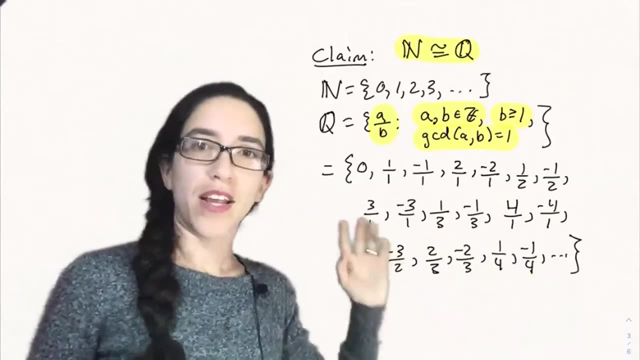 possibilities. in this case These are relatively prime, Negative 2 over 3,, 1 over 4, and negative 1 over 4, and that's sum equal to 5.. Then you list the ones that sum equal to 6, etc. Notice that. 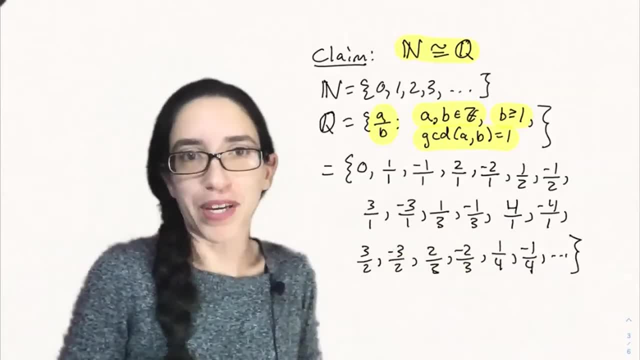 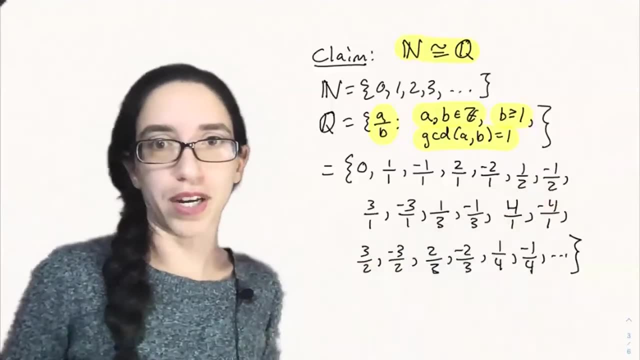 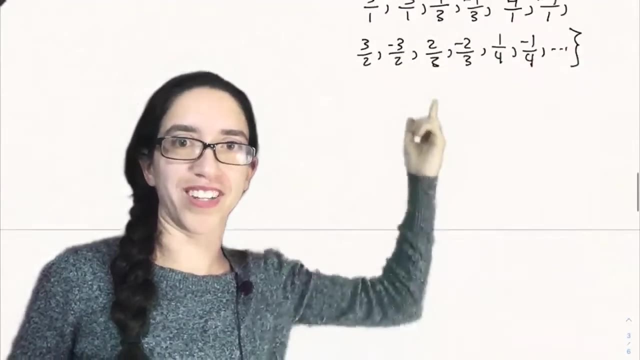 every single rational number is on this list. We didn't miss any, because every rational number has a sum of its numerator and denominator, and so it eventually is reached by this list. Then we can make the bijection where 0 maps to 0, and 1 maps to 1 over 1, and 2 maps to minus 1 over 1, and so on. 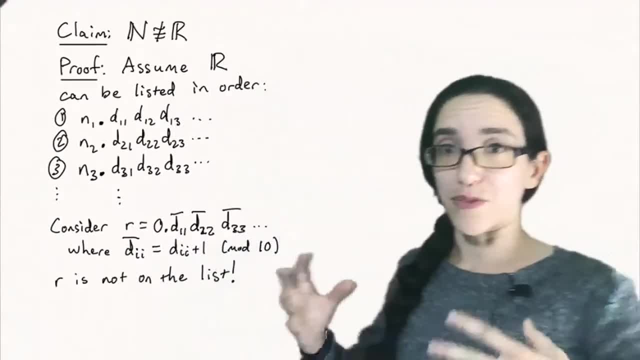 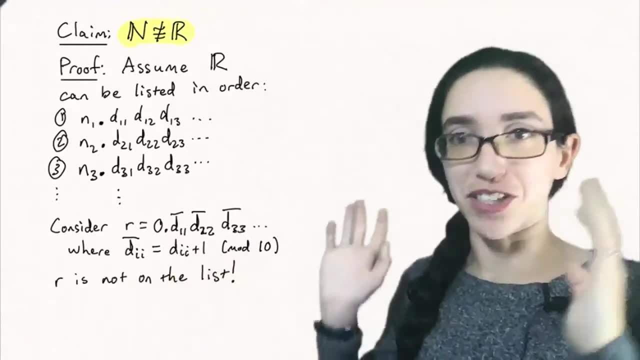 because we listed them in order. The natural numbers and the rationals have exactly the same size, but interestingly, the natural numbers and the reals do not have the same size. The reals are actually a bigger size of infinity than all the three sets we looked at before. The proof of this: 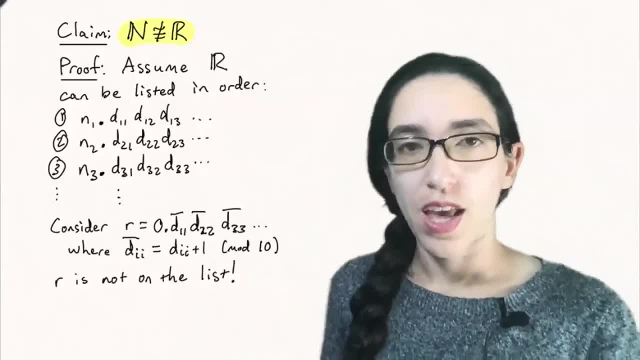 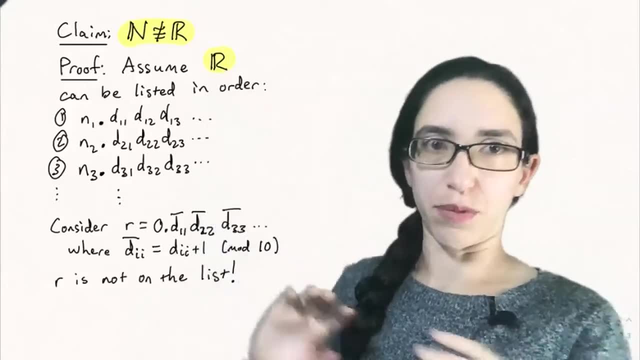 is a classic proof by contradiction. It's called Cantor's diagonal argument, and the proof by contradiction says: we're going to assume it's true and show that something goes terribly wrong, so let's assume that the real numbers can be listed in order. That's what we need to have a bijection. 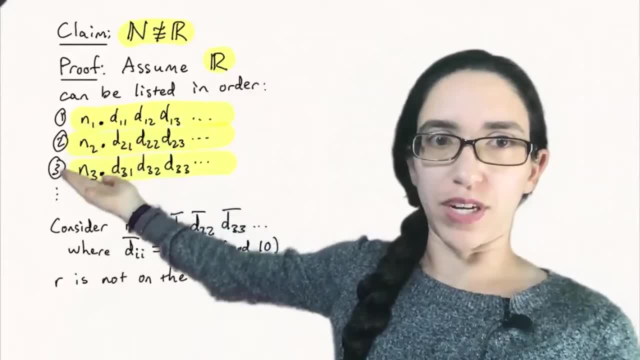 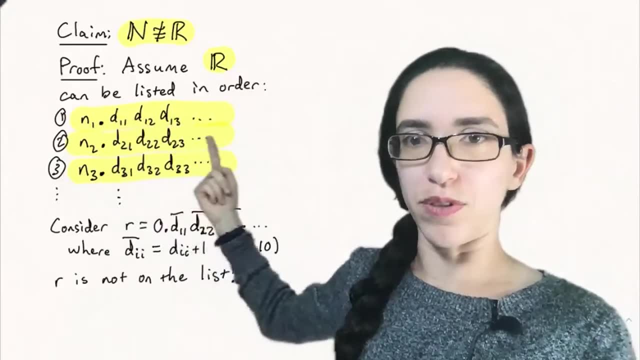 with the natural numbers, so let's list them as some integers: n1,, n2, n3, point, and this is in decimal form. so d11, d12, d13, etc. are just decimal digits between 0 and 9, so this is writing. 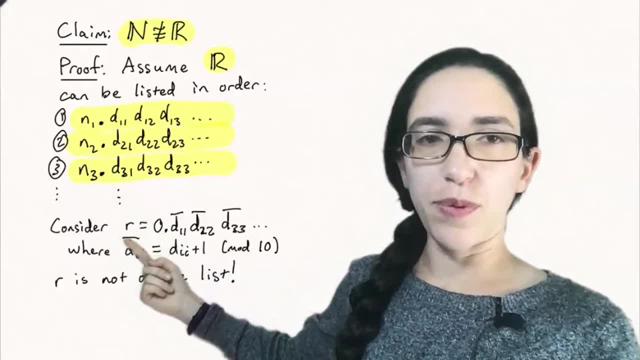 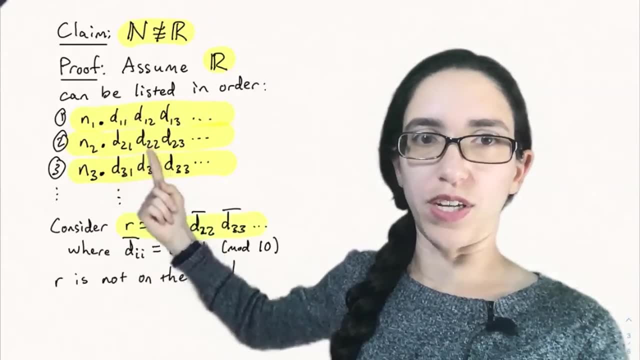 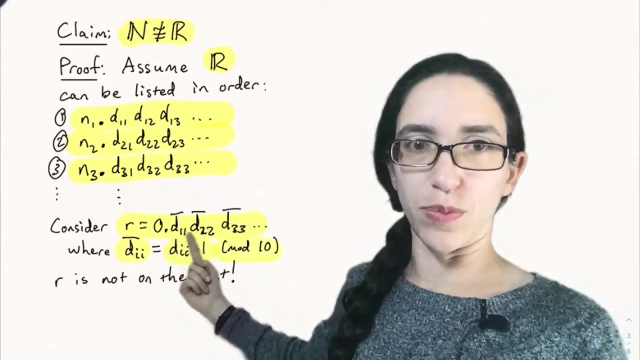 numbers 1,, 2,, 3,, 4,, 5, and now we consider the number formed by changing each of the diagonal digits. so take d11,, d22, d33, take the diagonal and make a new decimal where you change each digit. 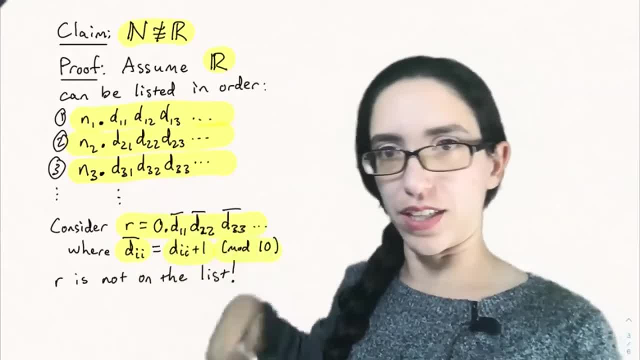 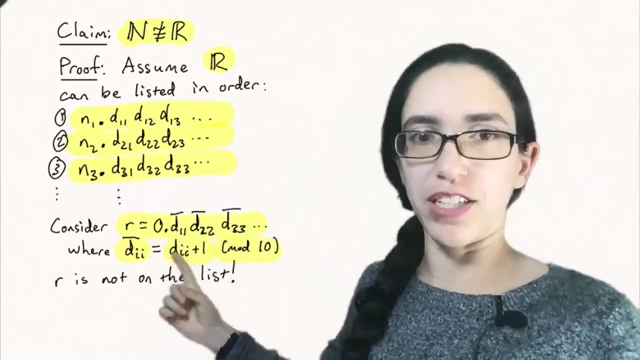 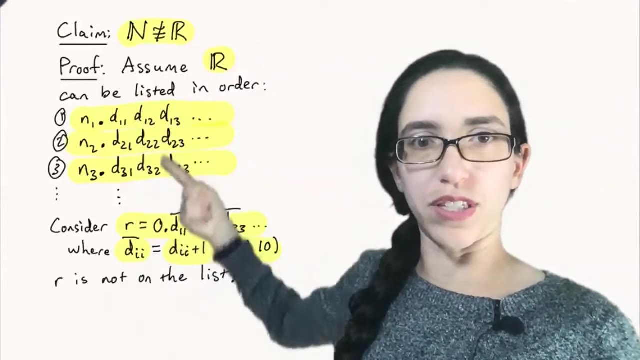 where d11 hat is, you add 1 cyclically, wrapping around mod 10.. You have to worry a little bit sometimes with 0.9 bar formats, but there's always a way of changing all these digits so that you can make this curve work. So this was true, and now we've got a new number and this number can't be on. 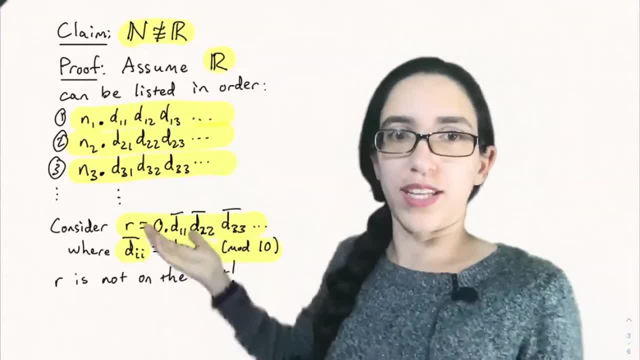 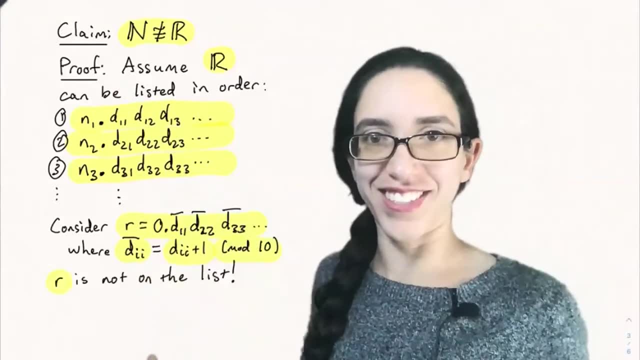 this list because it's different from every one of these numbers in the list by some dii because we changed each of those diagonal elements and that gives us a contradiction. because we said that we list, that we assumed that we listed all real numbers and we created a real number out of that.